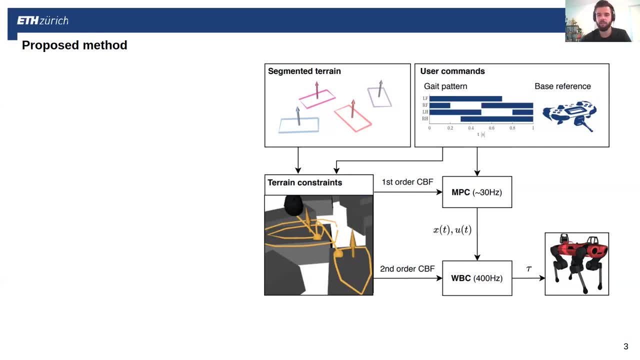 Those two together form the terrain constraints around the normal nominal gates, and these terrain constraints are to be fed into both of the control layers. So, as the planner, we have here a model predictive controller which uses a simplified model And by having a horizon, it can reason about dynamic locomotion and terrain constraints. 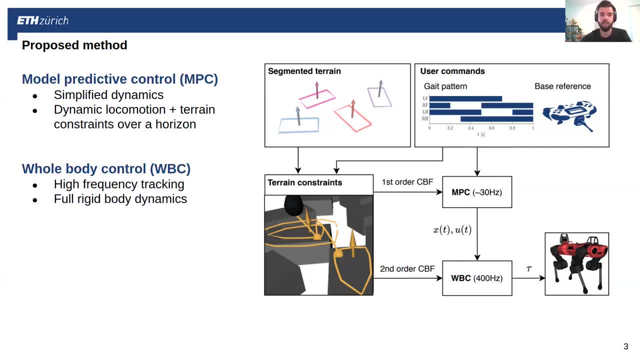 across this horizon. As a tracking controller, we have a whole body controller which executes at a high frequency and decides the torque based on the full rigid body dynamics of the system. And finally, we propose to use control barrier functions to tie it all together. 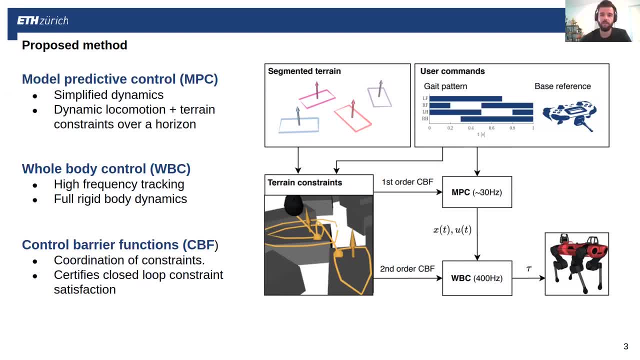 So this will be the method that translates the terrain constraints into concrete constraints for the MPC and whole body controller And in the end it will also serve to be a certificate that will show us that the closed-loop system actually will satisfy the terrain constraints. 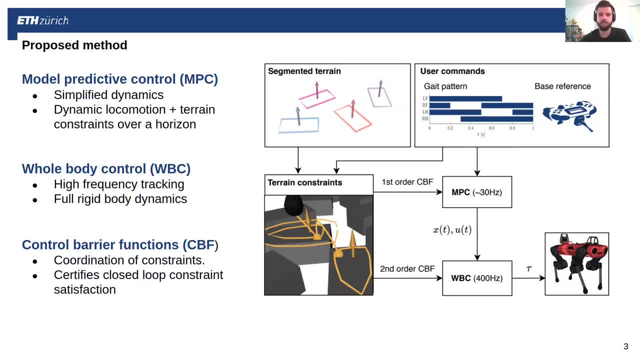 This slide then also gives the agenda for this talk. So first I'll start discussing the model predictive controller and whole body controller and afterwards we have to choose a way to build it. we'll move on to the control barrier functions and see how they tie in. 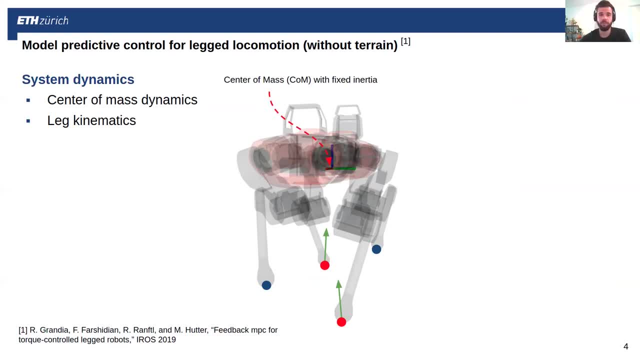 First of all we have the model predictive controller, which builds on our previous work. For the dynamics we assume a fixed inertia around the center of mass and we consider the legs only kinematically. So that gives us the 12 center of mass states. 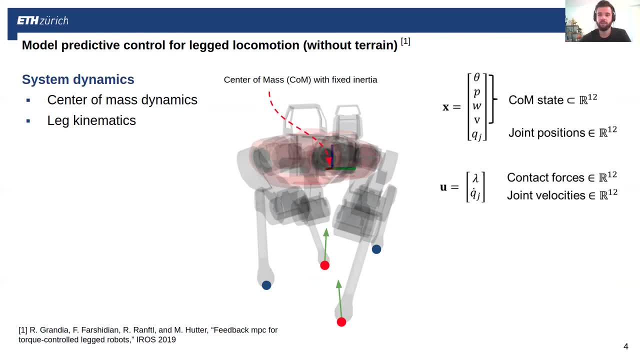 and joint positions And as control inputs we have contact forces at the feet and the joint velocities. Over that model we pull some constraints. So for stance legs we want it to be zero foot velocity and the contact forces need to be within the friction cone constraint. 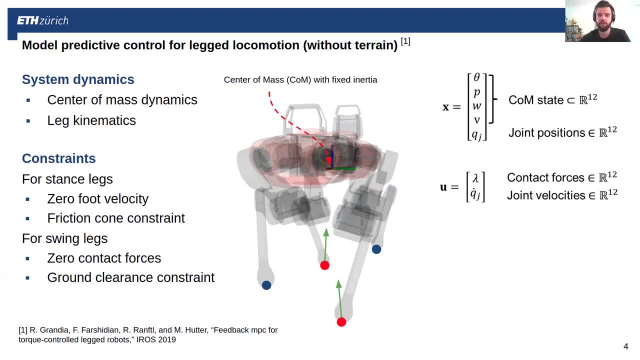 And for swing legs we require zero contact forces and some ground clearance. And these constraints are then posed based on the predefined gate pattern. So the MPC doesn't alter the gate timing. It actually thinks of the whole body control as an indicator of the dynamics itself. 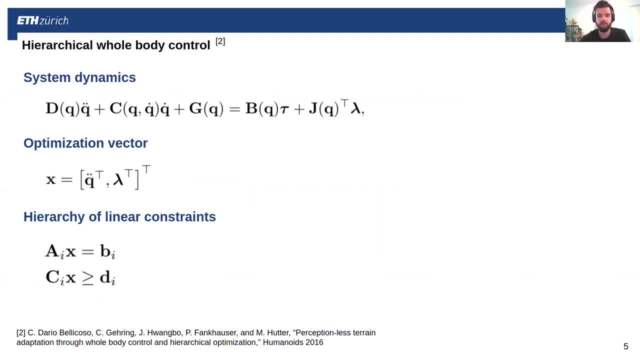 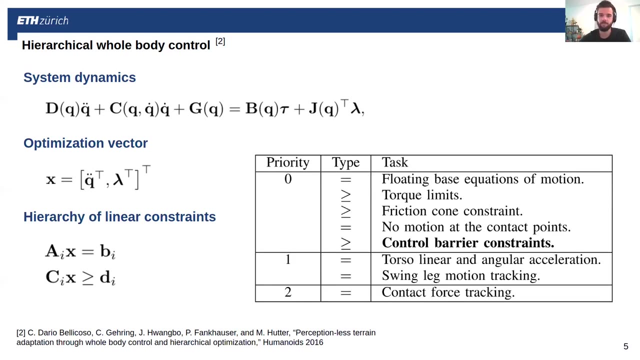 Moving on, we have the hierarchical whole-body controller which considers the full nonlinear dynamics of the robot and it creates an optimization over generalized accelerations and contact forces. Then we're able to impose a hierarchy of tasks which are specified through equality and inequality constraints. 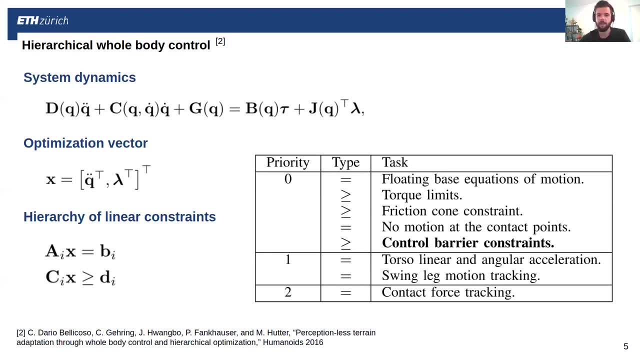 And in this work we have at the highest priority basically- and to that set we'll add also the control barrier constraints which are introduced later. Below that we have the tracking constraints, so tracking the desired reference for the torso and the swing legs, and at the lowest priority we have contact force tracking, which then regulates. 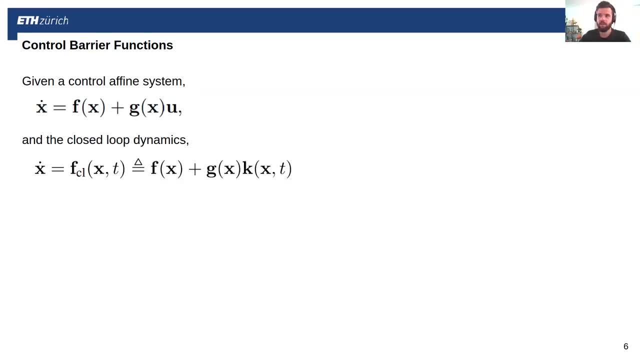 the internal forces between the feet. Then on to the control barrier functions. For the precise mathematical definitions I would like to refer to the paper and the references therein, but for this talk I would just want to give some intuition of what's going on, Starting with a control find. 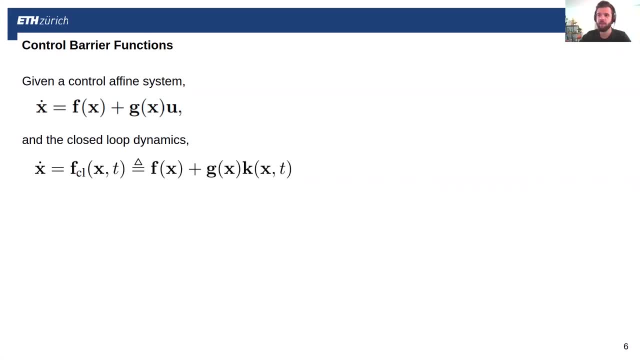 system and, after plugging in our controller k of x- t, we'll create some closed loop dynamics and what we're going to do is to think about the safety of a set with respect to this closed loop dynamics, and the set is, in this case, defined through a function h of x, of t and the interior. 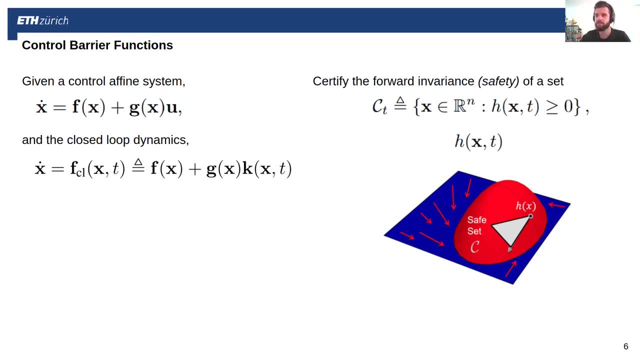 of the set will be wherever this function is greater than zero. Now what we want from our controller is that it renders this set forward invariant under the closed loop dynamics, meaning that if we start inside, we are guaranteed to remain inside for all future time. and additionally, what we would really like is if we 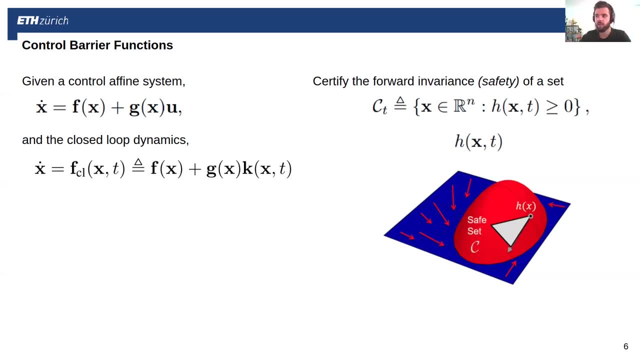 do happen to find ourselves outside of the safe set, we want that the controller makes a reasonable effort to get back to the interior, and this can all be achieved through what is called the control barrier function. This gives us a sufficient, point, wise and time condition that tells us how to pick. 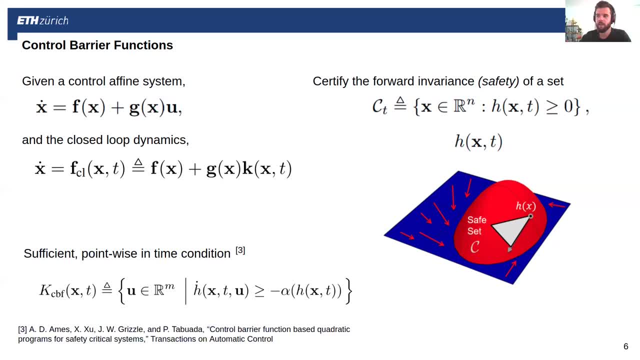 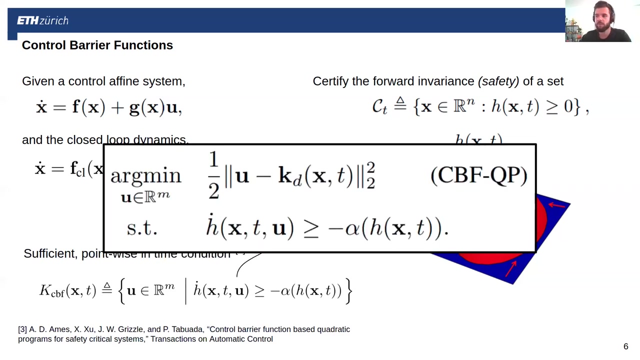 all inputs that satisfy the safety requirements. and this constraint requires that we make the time derivative of h bigger than some negative scaling factor alpha of the original function h And we see how the control input u enters through the dynamics, this time derivative of the barrier function h. Now this theoretical framework has led several practical controllers in the literature. 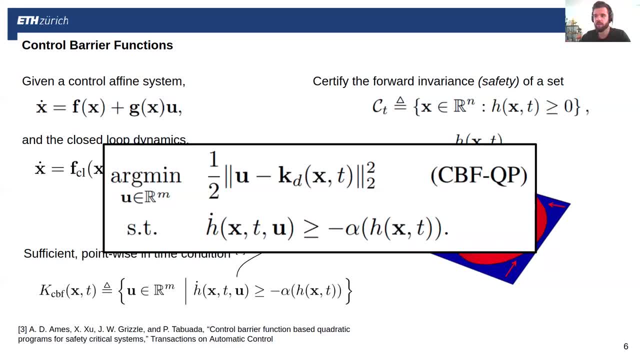 and a popular one, is the CBFQP. as shown What it does, it takes a reference controller, kd, and it tries to find an input that is as close as possible to the reference while at the same time satisfying the CBF constraint. We will use this controller as well as a baseline in our results. 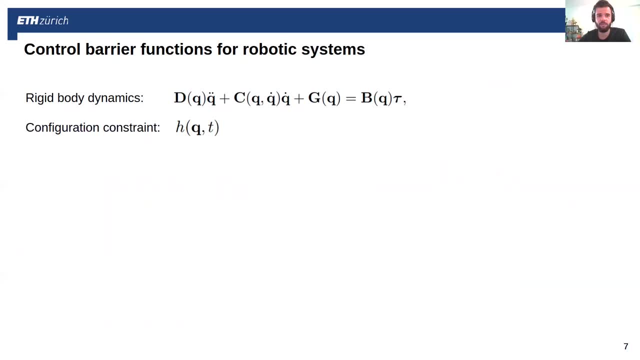 Then, speaking more concretely about CBFs in the context of robotic systems, we have here the rigid body dynamics and we would like to put some constraints over the configuration of the robot. Then, when we take the first order- CBF- we get a condition over the velocity, basically, of the 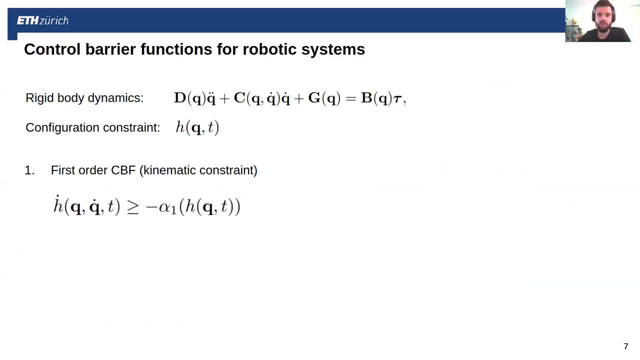 robotic system. So if you want now a condition with respect to the torques, we have to do some more work, And what's done there in the literature is what is called an exponential barrier function. So it takes the first barrier function as a new equality constraint. 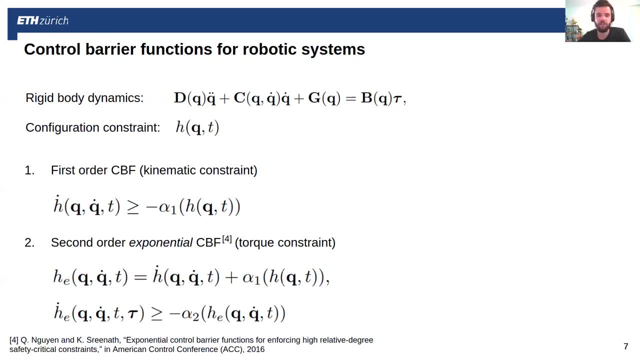 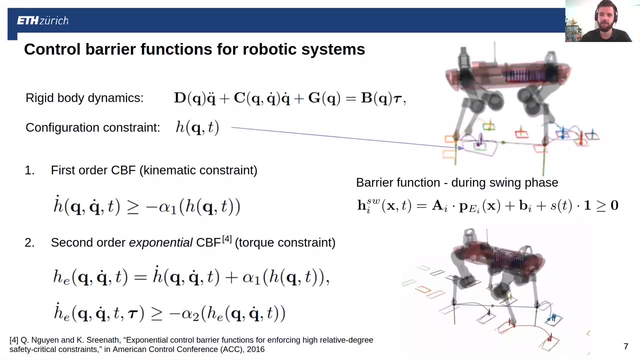 and then places an additional barrier function over this extra constraint, Now satisfying this second order. CBF is then also guaranteed to keep us within the original safe set In the context of our stepping stone problem. the configuration constraint is as follows: We define the barrier through the projection of the foot on the target plane and create a shrinking. 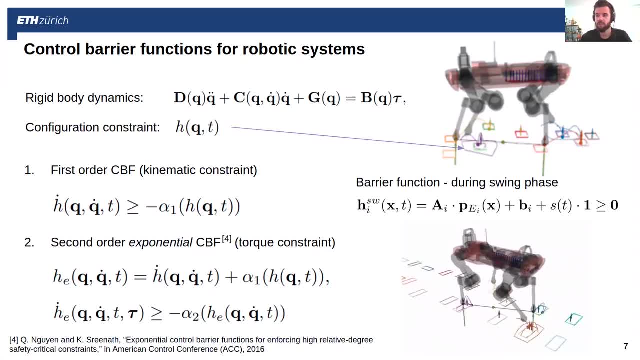 set of half spaces. This shrinking set is, in this case, the safe set and it will shrink to lie on top of the stepping stone towards the end of the swing phase. Staying within this safe set thus guarantees that we end up on top of the stone And from that single configuration constraint we 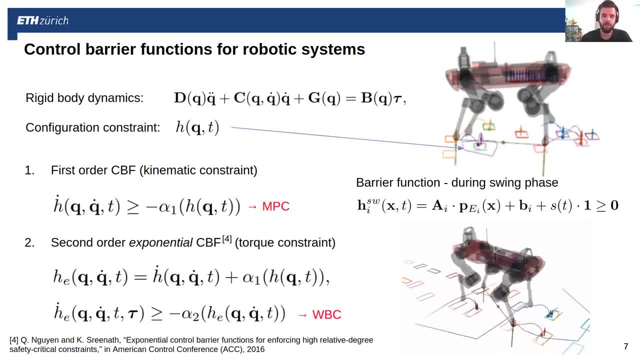 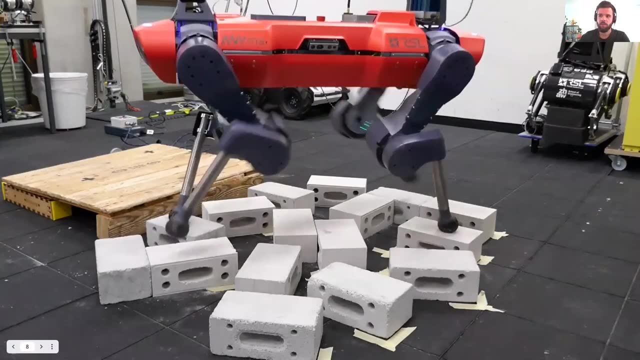 can derive the two CBFs. The first one, the kinematic one, will enter the MPC and the torque level constraint will enter the whole body controller. With all the constraints defined, we can move on and see how this setup performs on hardware. Here we have initialized the robot. 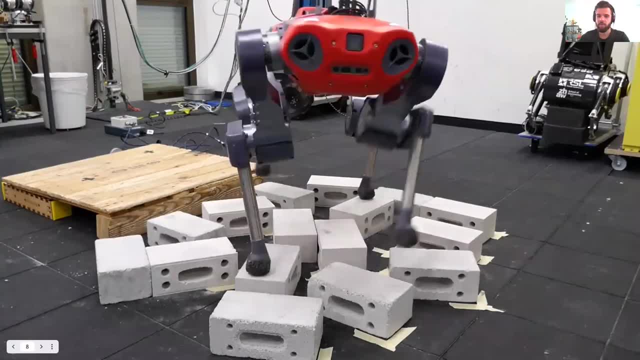 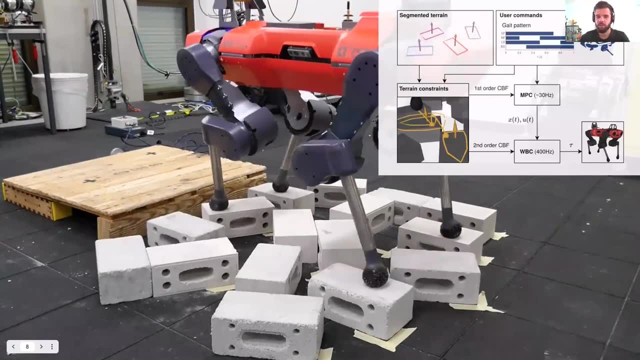 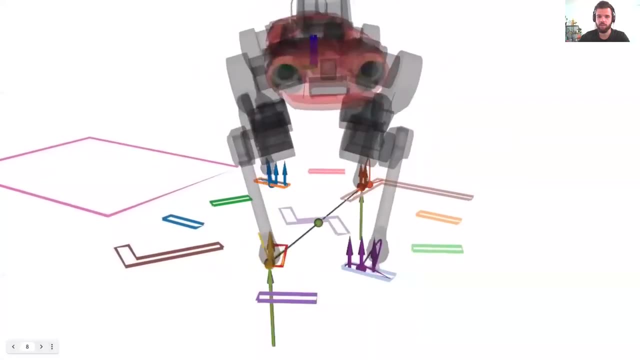 on a pre-mapped environment and from there we command it to trot. Basically, give it some velocity commands. From those input it autonomously decides on which of the stepping stones to step and through the MPC it decides which location to step exactly. Then the whole body controller ensures that this plan is executed with a high quality. 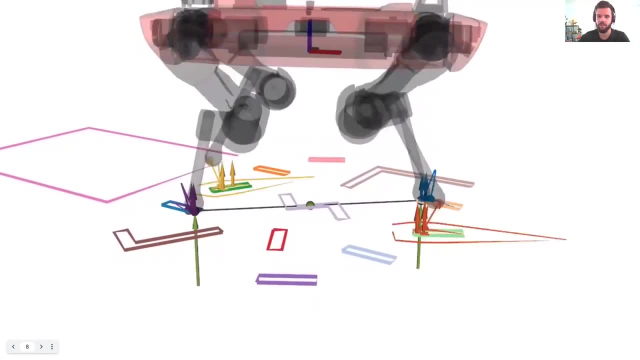 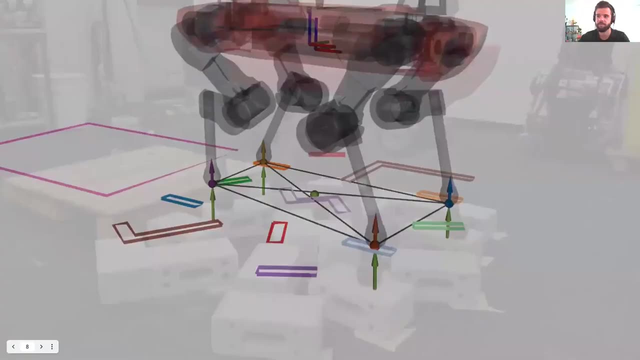 Showing here the internal state of the MPC. we see again the various safe sets as they appear during each of the swing phases to ensure that we land on the next stepping stone. As we move here on to the next platform, we see how the controller coordinates the base and 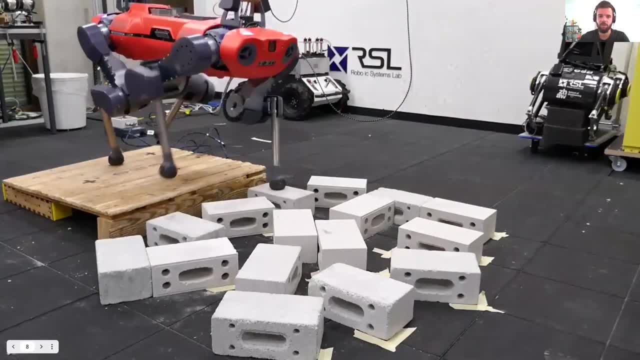 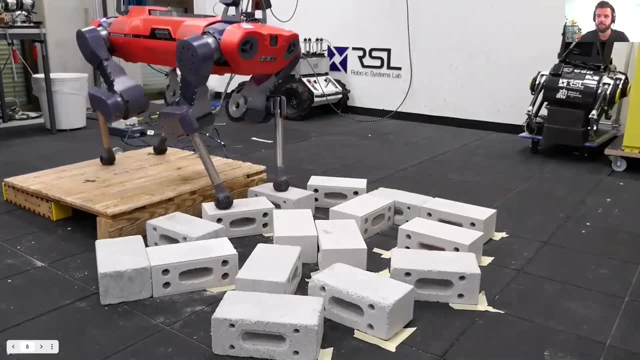 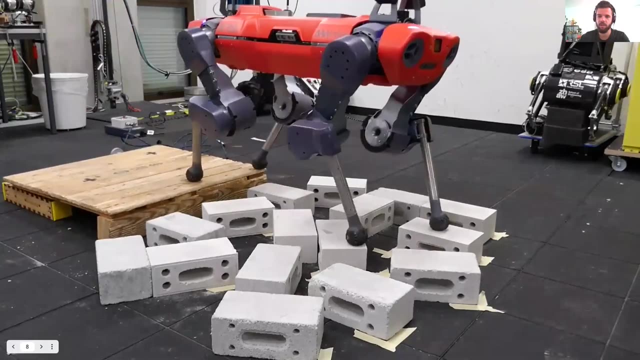 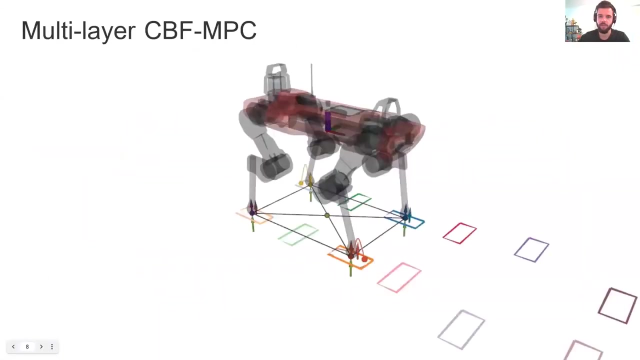 stepping locations to achieve this dynamic locomotion across the environment, And because doing a detailed comparison between different controllers on hardware is quite difficult, we also do some more controlled simulation studies to compare the difference between different methods. Here we first have the proposed method, navigating our stepping stone. 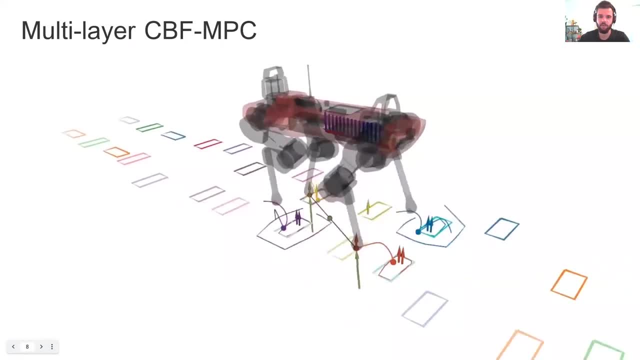 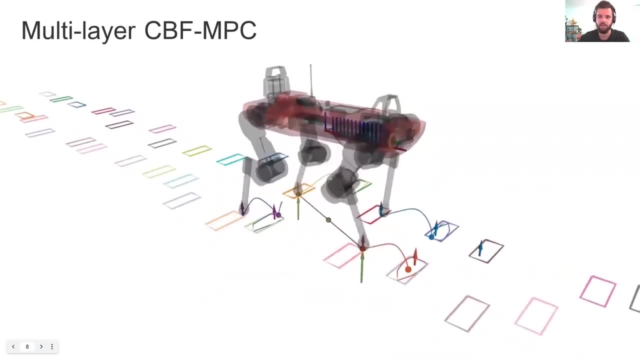 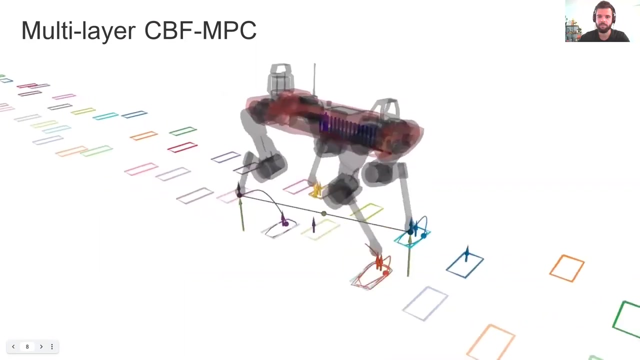 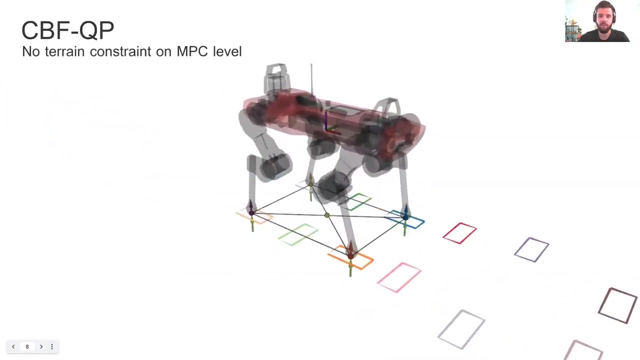 scenario where the stones are randomly spaced in a forward direction. We give the controller here desired velocity of 0.25 meters per second and keep this velocity constant until it reaches the end of the scenario. You can now compare this to the CBFQP approach, which only has the terrain constraints in. 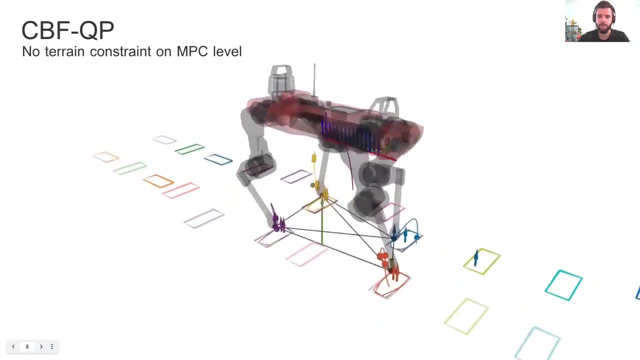 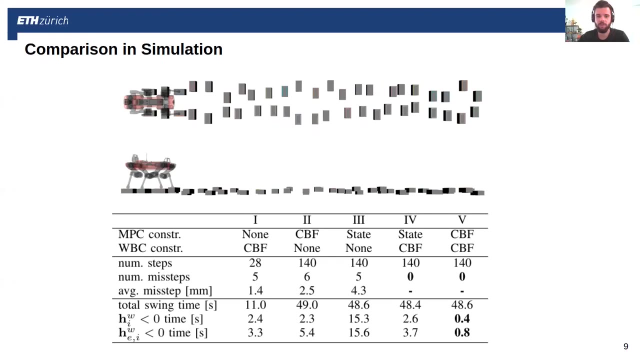 the lowest filter of the controller. So we saw that the CBFQP controller does well for a few steps but then quickly falls when the scenario becomes more difficult. We can have here a more detailed look at what was going on. So here on the left we have controller one which was the CBFQP, and it doesn't have any. 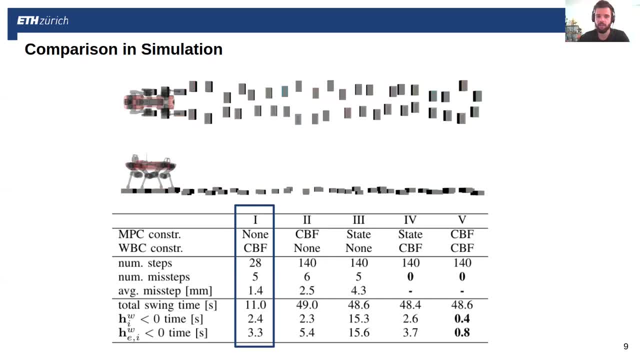 terrain related constraints in the NPC and it only has it in the tracking controller basically. So that's the reason that it satisfies the terrain constraints quite well for the first few steps, but then it lacks this long-term horizon to coordinate dynamic locomotion and 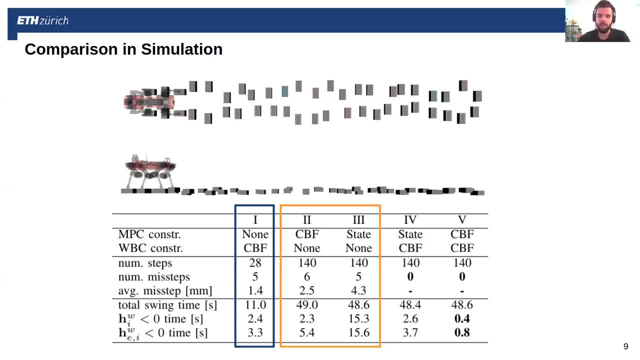 the stepping constraints together. Then as a second group of controllers we can compare to controllers that have constraints only at the NPC level. So controller two has them as CBFs and in controller three we formulate them differently as state constraints. So this is basically an inequality on the landing location of the foot. to be on top. 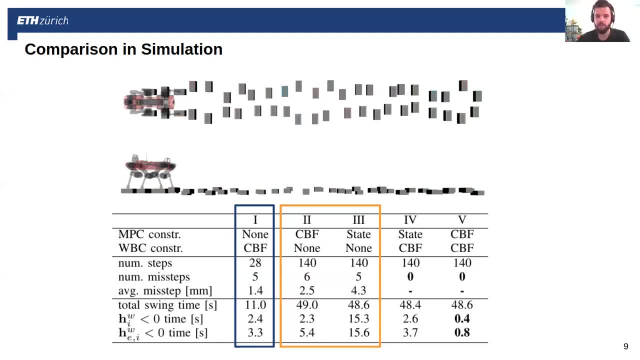 of the stepping stone And we see that both these controllers reach the end of the scenario, but both of them also have some mistakes, So we record how many times they step just outside of the boundary of the stepping stone and by how much. So we can do better. and we can do better by including terrain constraints as well in. 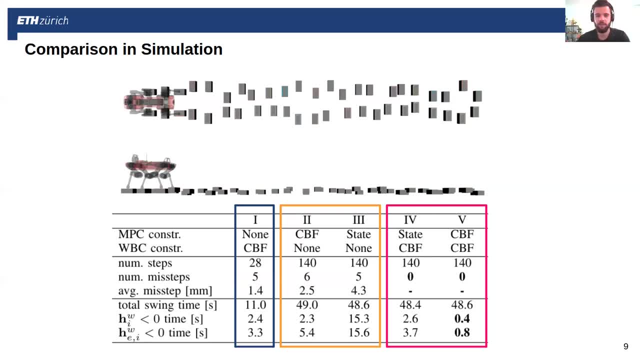 the tracking controller. So these last two controllers now have terrain constraints both at NPC level and at tracking level, And number four has it as state constraints and number five- our proposed method- has it as CBFs on both levels, Both these controllers. 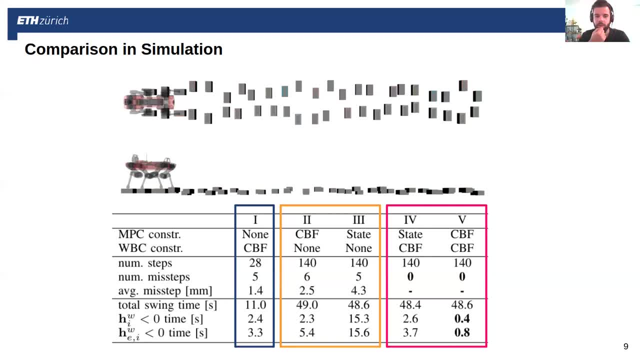 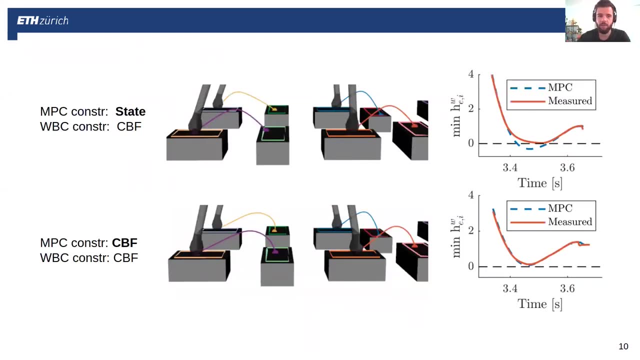 achieve the full scenario without any missteps. but when we compare them on the safety metric- so how often do they exit the safe set- we see that controller number five spends the least time outside of this safe set. And to have a more detailed look to see why that happens, we look here at the first swing. 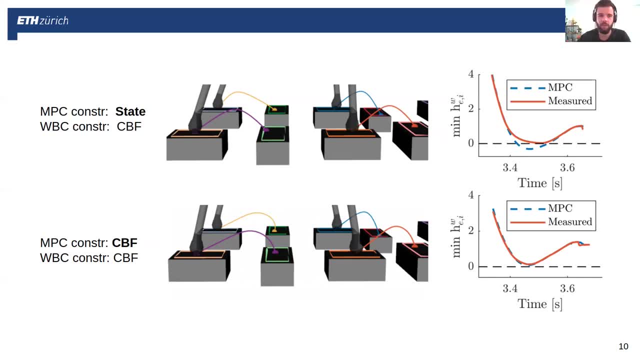 phase of both controllers. So the top one, we have the one with NPC state constraints, and then the bottom one, the CBF constraints. So you'll notice that they have a very different swing plan for the upcoming swing phase And this is confirmed in the graphs on the right. 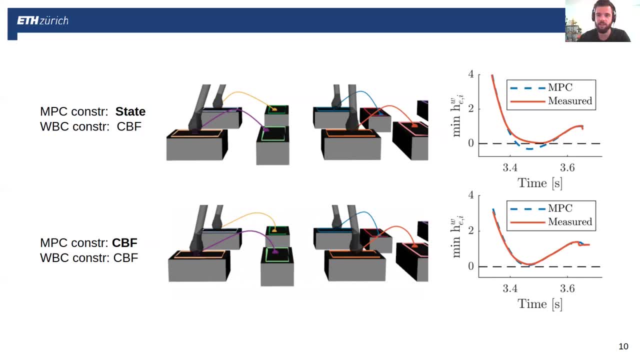 So we plot there the plan of the NPC with respect to the safe set and then the executed one where the whole body controller has executed the plan. So on the top we see that the NPC does in the end land within the safe set. but because 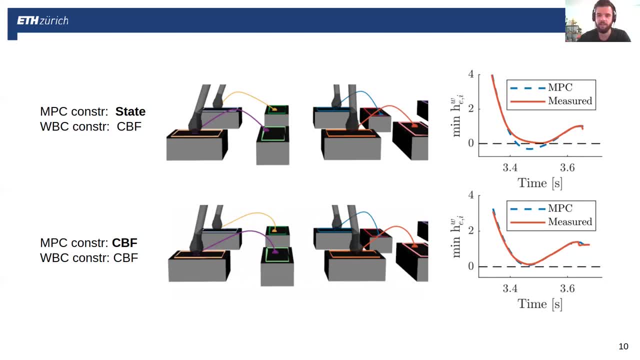 it doesn't have the CBF constraint, it exits the safe set In the middle of the swing phase And then, because the whole body controller does have the CBF constraint, it is forced to deviate from the plan. And finally in the bottom we see when both have the CBF derived from the same constraints. 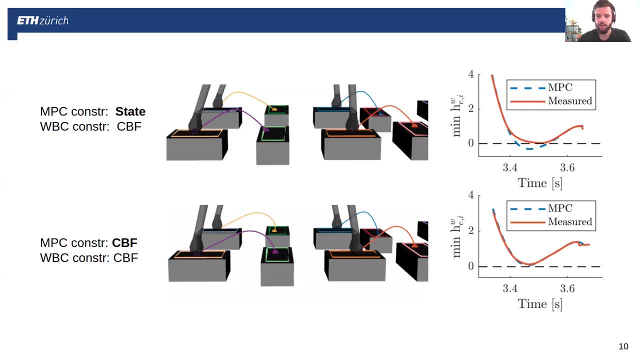 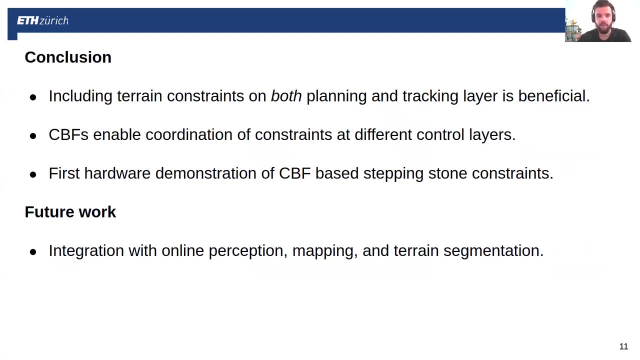 they are consistent and the plan and the executed swing trajectory are very close. So, in conclusion, we can say that including terrain constraints on both planning and tracking level is beneficial, And CBFs are a great way to coordinate the constraints that you can formulate at these. 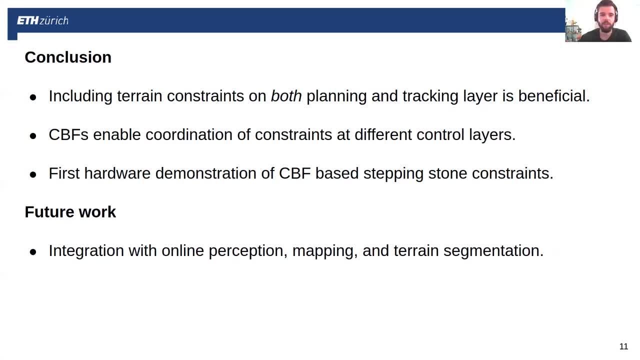 different layers. Additionally, we want to note that this is the first hardware demonstrations of using CBF to solve this stepping stone locomotion problem. We think it's really important to add this additional planning layer, because most of the references have only used the CBF QP controller. 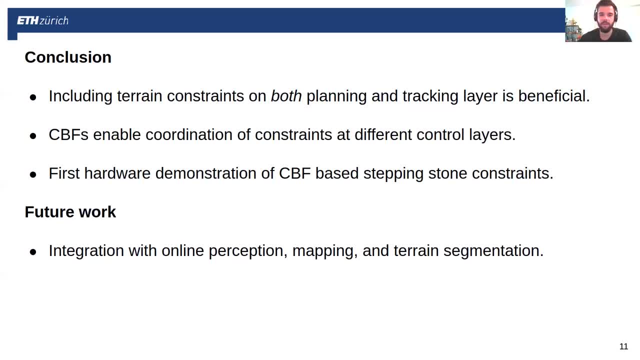 Finally, for future work, we would like to integrate this pipeline now with online perception, mapping and terrain segmentation, because in this work the terrain was still pre-mapped and we would like to do that online so we can send the robot into the wild.